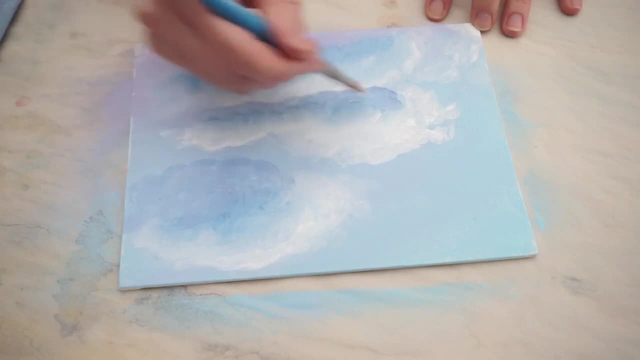 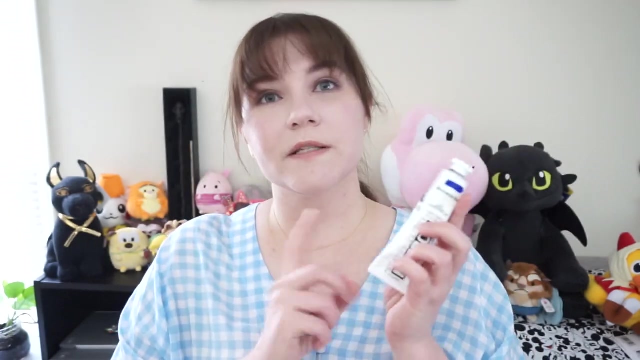 absolutely beautifully with and without medium, And because of their blendability you can get all the colors and the shades you want- kinds of really cool effects with them. Golden paints also thin out very well with water and thanks to their high pigment load you can get really 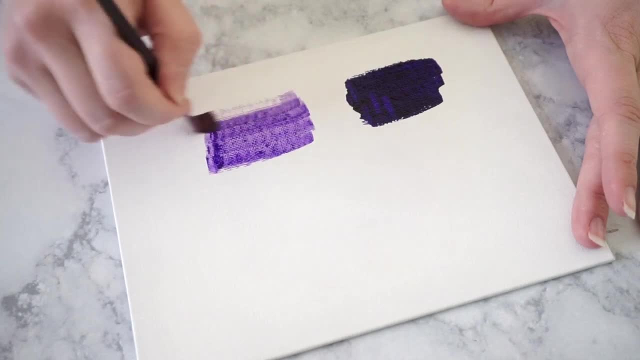 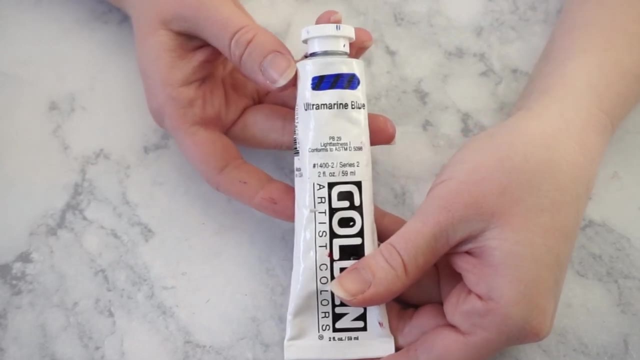 beautiful acrylic washes and you can even get some really beautiful watercolor effects. So Golden's packaging is really nice and they do actual paint swatches on the tube so you can see with more accuracy what the paint is going to look like. They have a lot of really beautiful colors on top of that. they 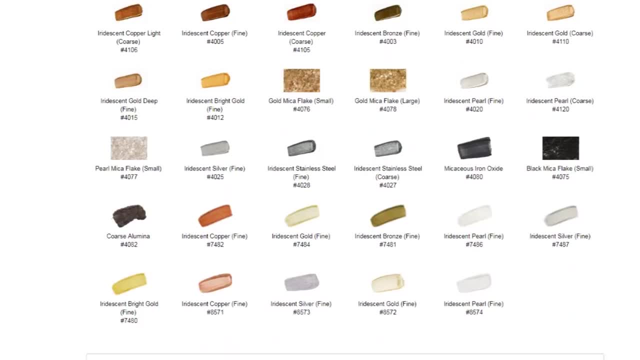 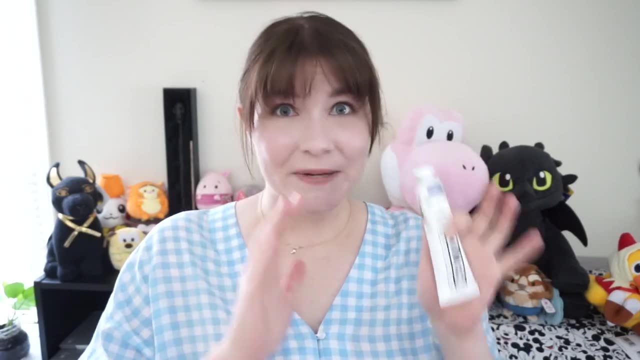 also have a line of iridescent colors that are beautiful. They're so nice. So now let's talk about the cons of Golden. Golden paints are pretty expensive. They can run as high as $15 for a 2 ounce tube and they can be even. 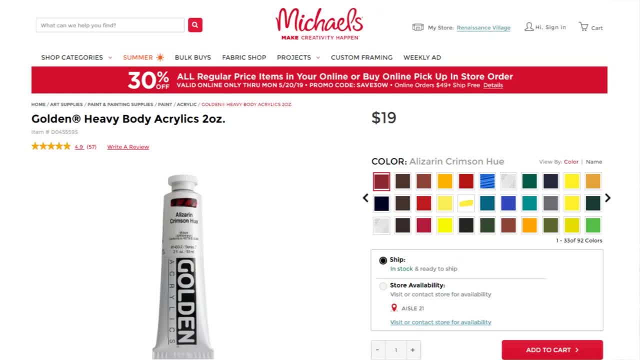 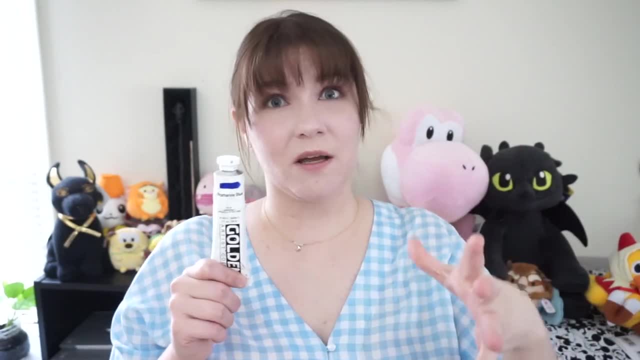 more expensive if you buy them at a craft store versus an art store. Golden paints dry really fast without a retarder or a constant mist of water, So if you forget to mist it like once, your paints basically gonna dry out. Last but not least, because of 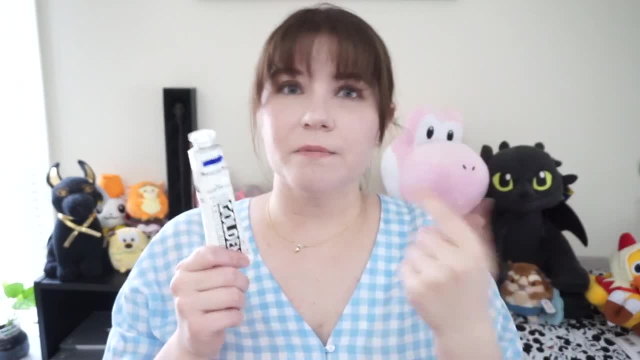 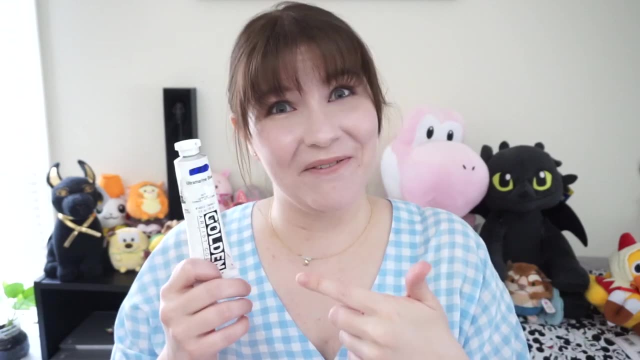 ắc, the high pigment load, which is a benefit, but because of it you can sometimes overestimate how much paint you need and therefore end up wasting paint. And this paint is kind of expensive, so you don't want to waste it, but yeah. 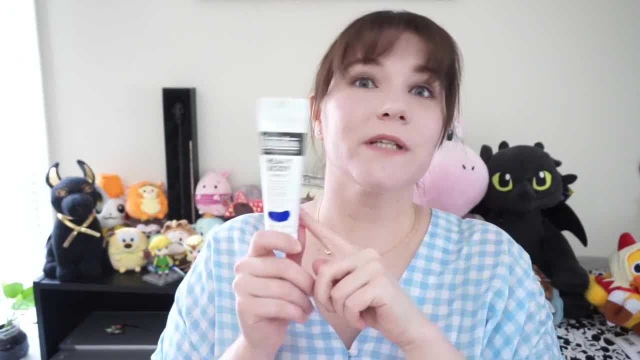 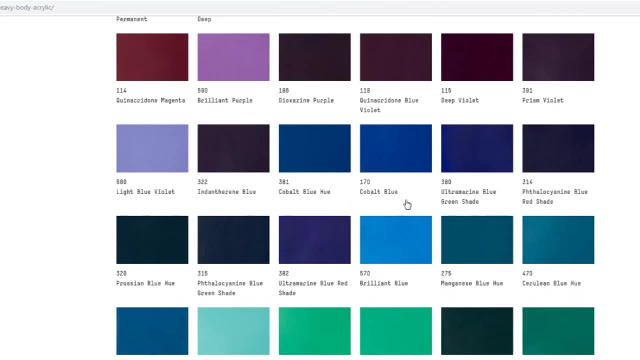 Alrighty, so let's move on to Liquitex's pros. Liquitex has a wide variety of colors, and they have something that they call their brilliant color line, which are basically neon. So that's pretty cool. So Liquitex holds texture really well. 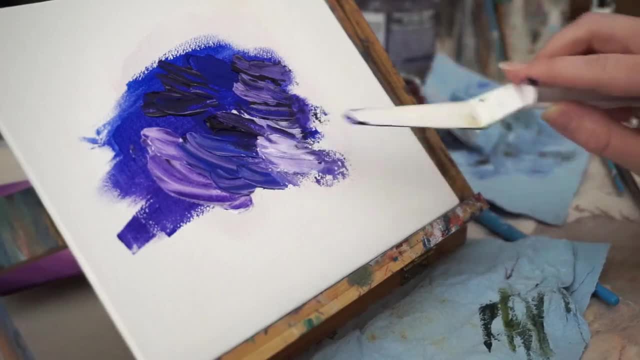 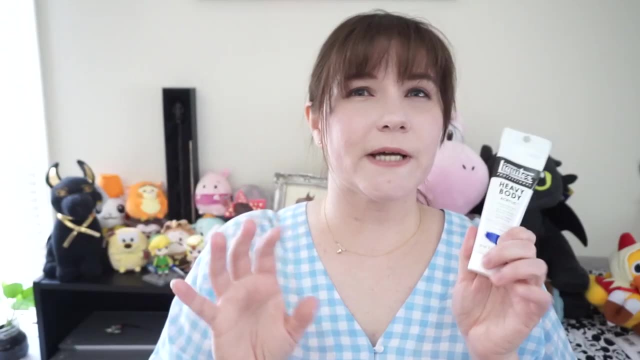 and it looks really great if you do bold strokes with a palette knife. Liquitex paints are actually decently priced for artist quality paints and they run a couple of dollars cheaper than Golden. Liquitex is also pretty opaque and they cover most services decently well. 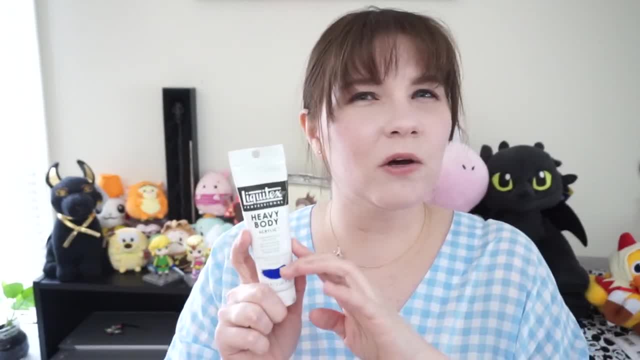 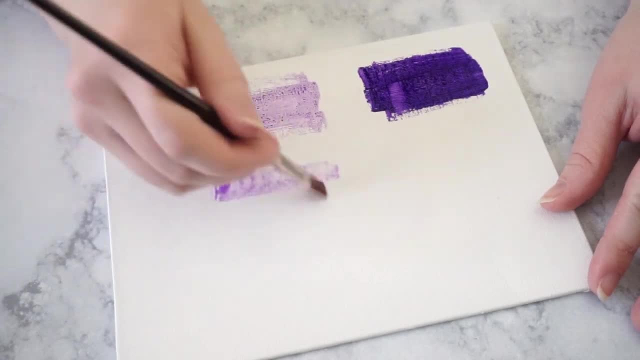 So let's move on to the cons. So Liquitex's pigment load doesn't seem to be that high. When you thin them out with water, they lose a lot of their color and saturation. The low pigment load also means that Liquitex 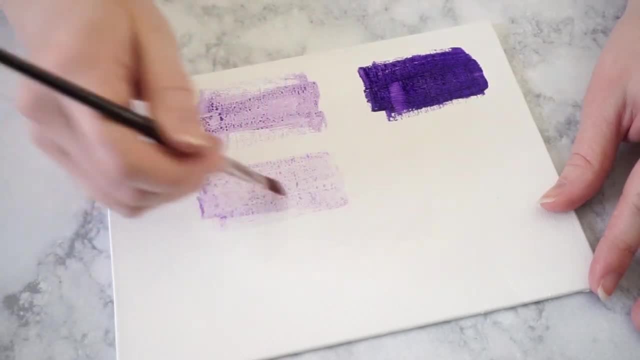 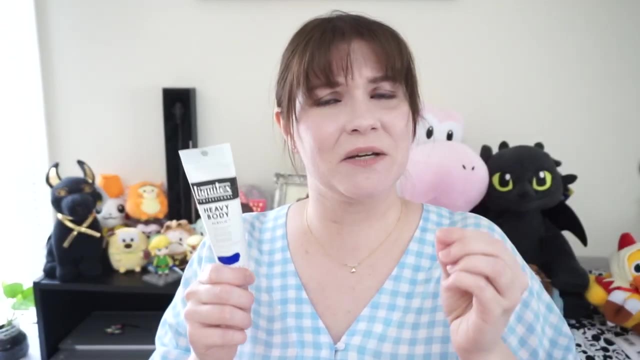 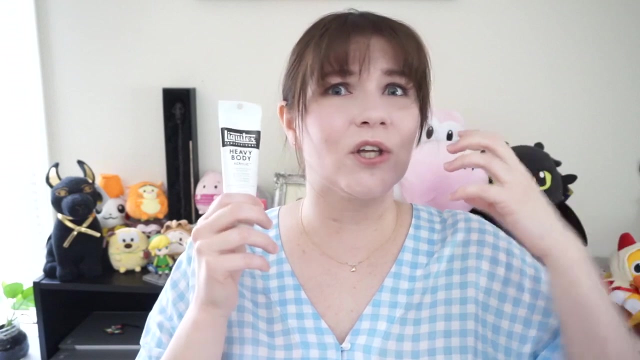 does not do acrylic washes very well. Oftentimes the colors are way too desaturated and the wash usually comes out uneven. The blending is also pretty inconsistent between colors. with Liquitex Some colors blend together absolutely beautifully and then with other colors it's a huge frustration. 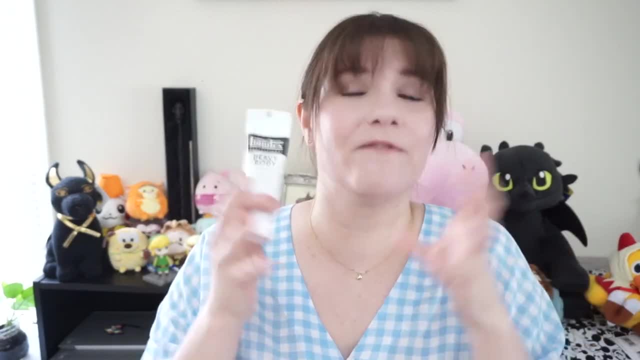 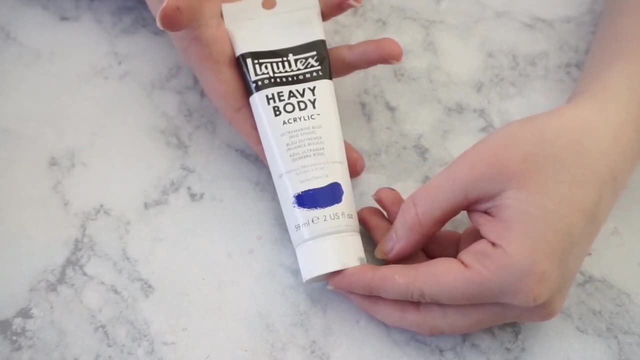 and fight to get them to blend at least decently well like, if at all. And lastly, the packaging. Instead of doing swatches on the tube, they just have a printed color swatch, which is really frustrating Because you can't tell what the paint is. 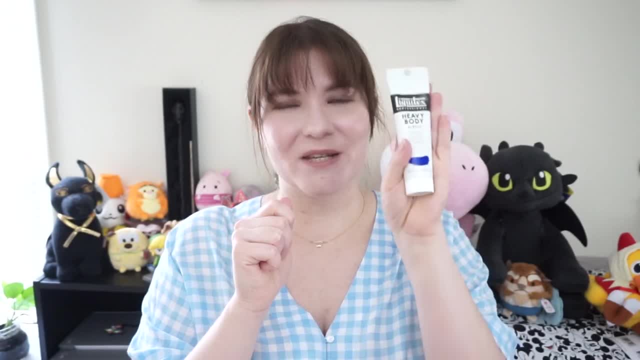 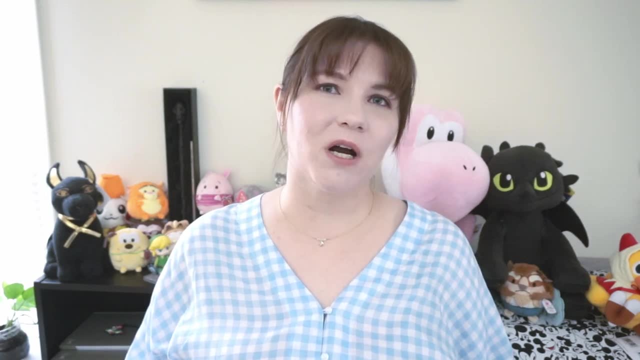 You have to physically open up the tube in order to see what the colors look like, because these can be drastically different from the paint inside the tube. So that was the pros and cons of each product, And between the two, the one I prefer the most is Golden. 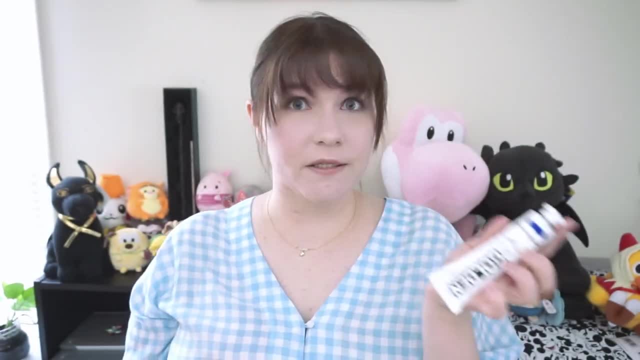 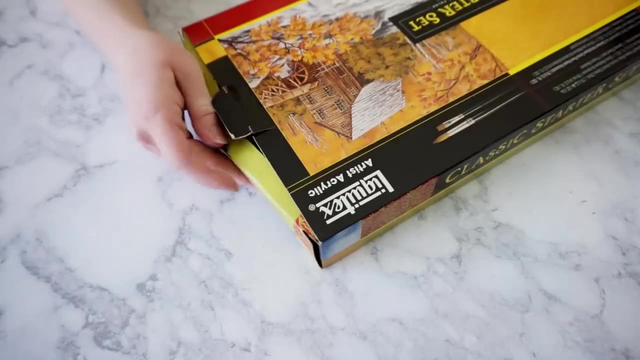 So I've been using Golden for a really long time and I've done dozens of pieces with it, So I'm a little bit more familiar with Golden than I am with Liquitex. So I bought a couple of tubes of Liquitex paint. 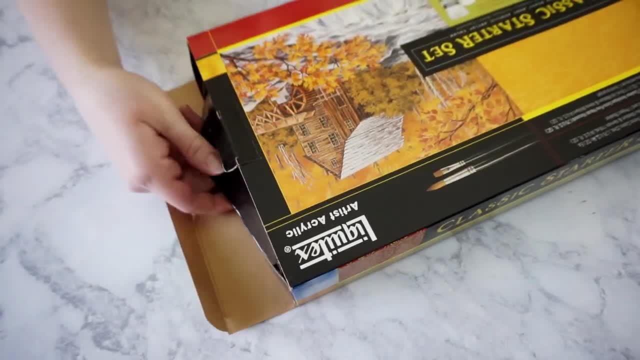 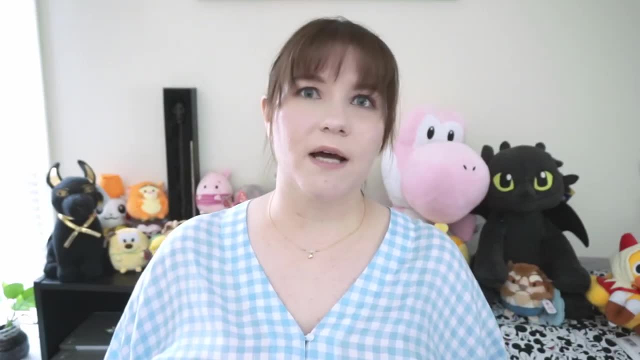 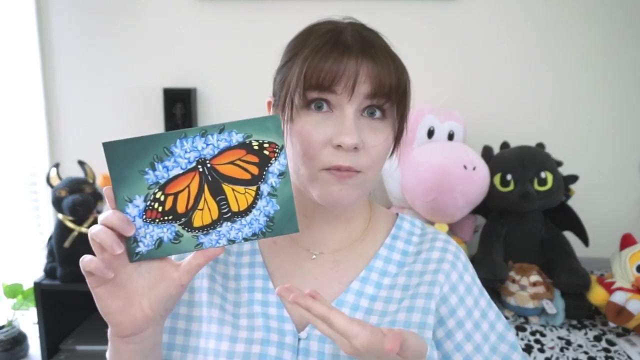 and the classic starter kit from Liquitex to test out the heavy body paints And I did a small Monarch butterfly study. I used my normal typical painting service, which is the Ampersand Gesso board, and I used a lot of my normal techniques with it. 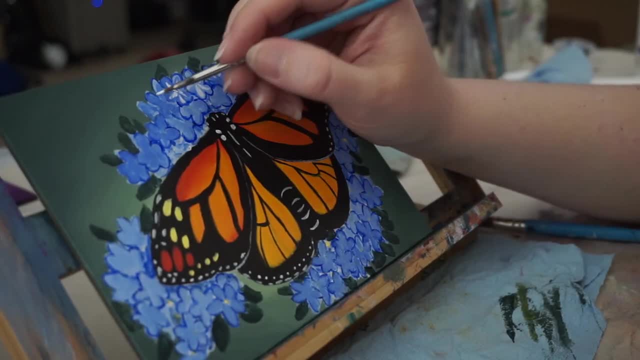 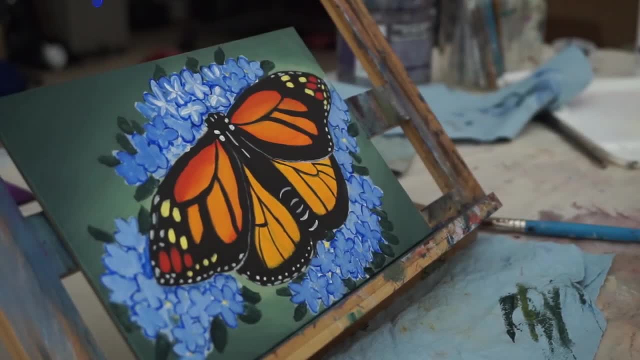 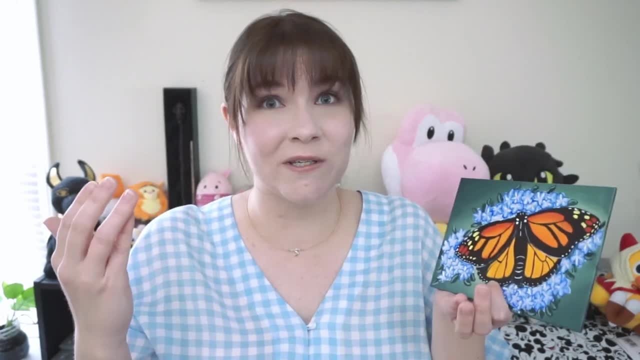 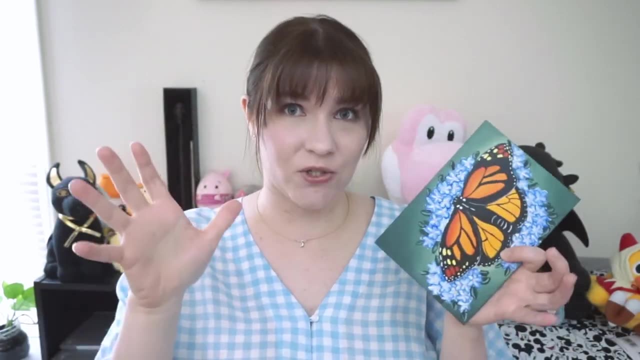 a lot of acrylic washes and glazes Because, guess what? It's excellent at holding texture and it's great for people who want to do a lot of abstract art or really graphic art and who want a lot of texture in their painting. Liquitex is excellent at retaining their texture.